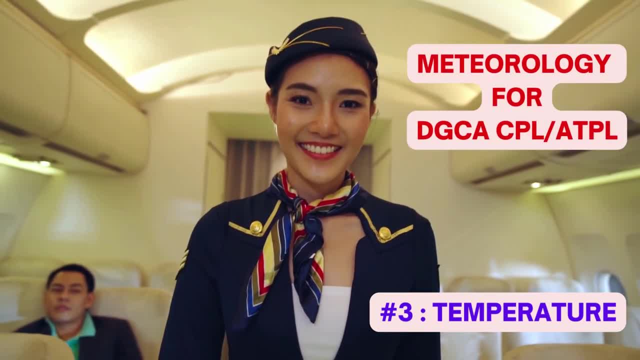 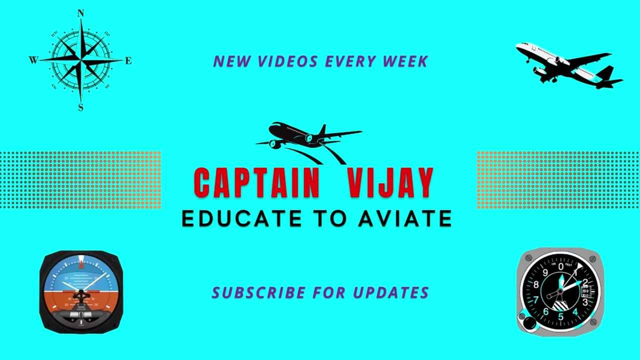 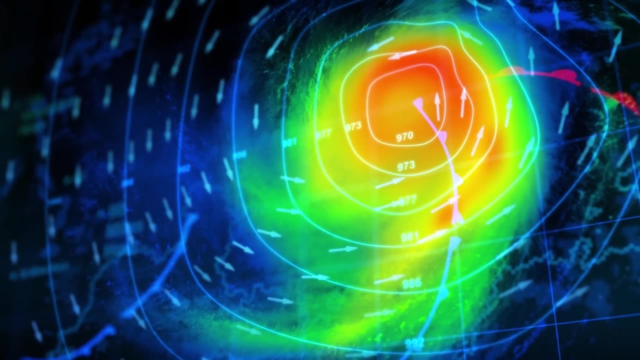 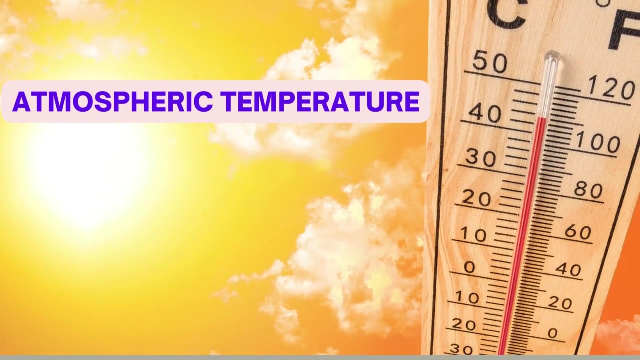 Hello everyone, I welcome you on board flight of Captain Vijay in the series of flights to study meteorology for DGCA, CPL and ATPL examination. Today we will fly through the third topic, which is temperature. So fasten your seat belts as we are ready for take off. 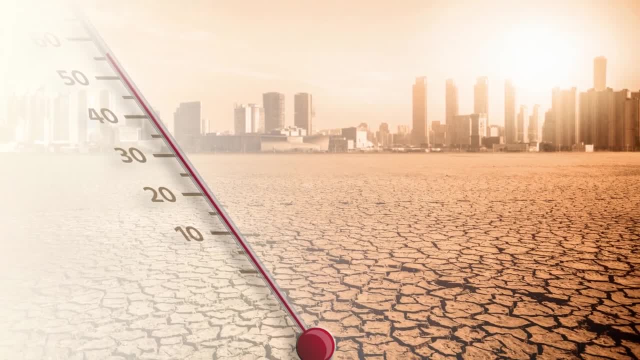 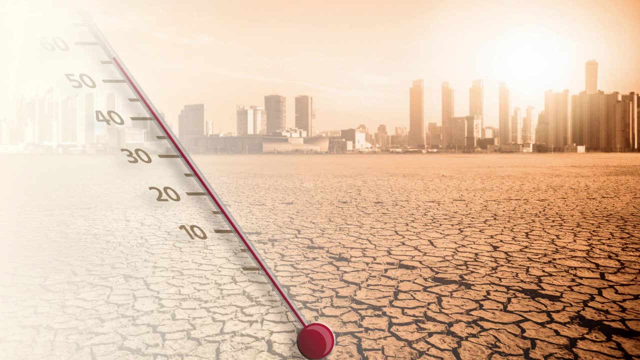 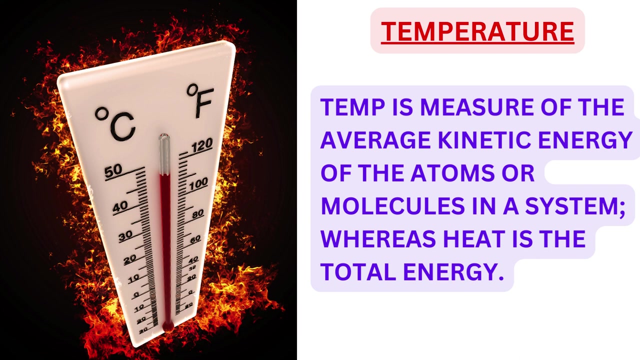 In the last flight we studied atmospheric pressure. After pressure, temperature is the most important variable in meteorology. Remember: information or data covered in this video under red outline is to be remembered for the purpose of examination. So what is temperature? Temperature is a measure of average kinetic energy of the atoms or 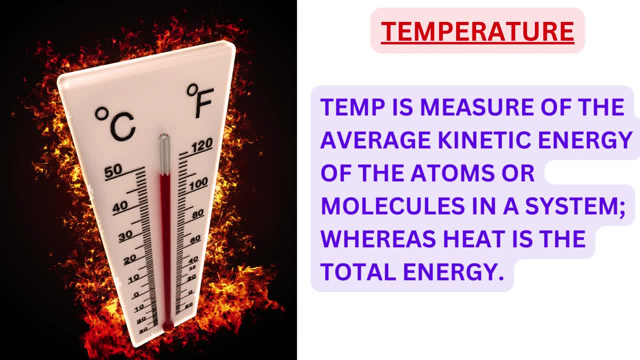 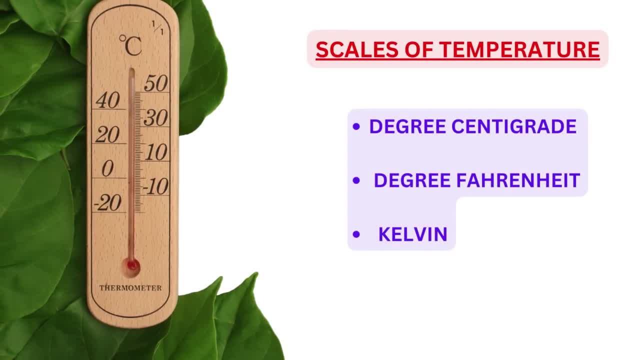 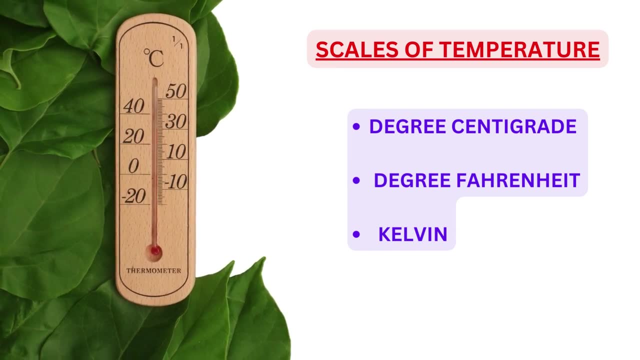 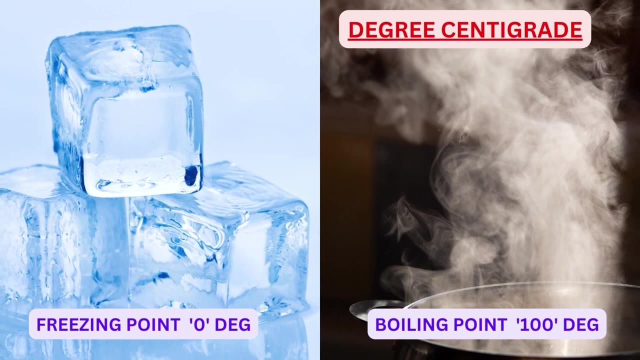 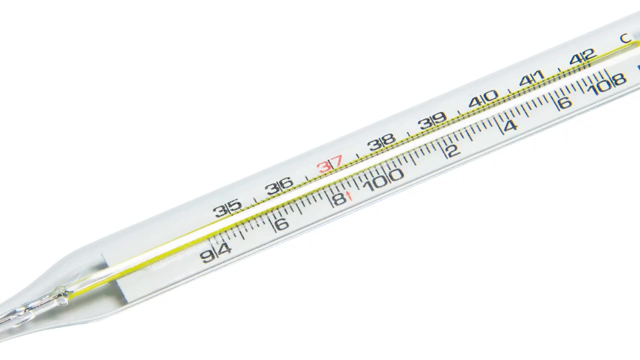 molecules in a system, Whereas heat is the total energy, And both temperature and heat are different. Temperature is measured in one of the three scales, That is, degree centigrade or degree Fahrenheit or Kelvin. Degree centigrade: you know very well, Water freezes at 0 degree centigrade and boils at 100 degree centigrade And in 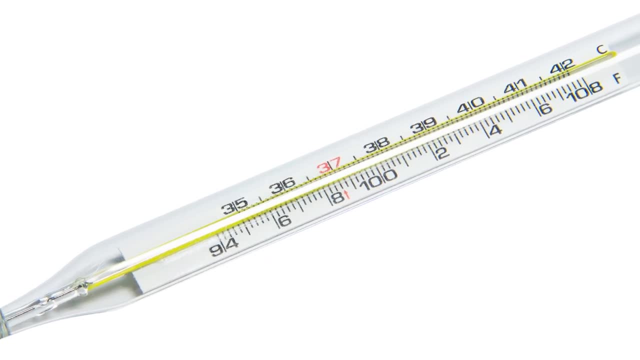 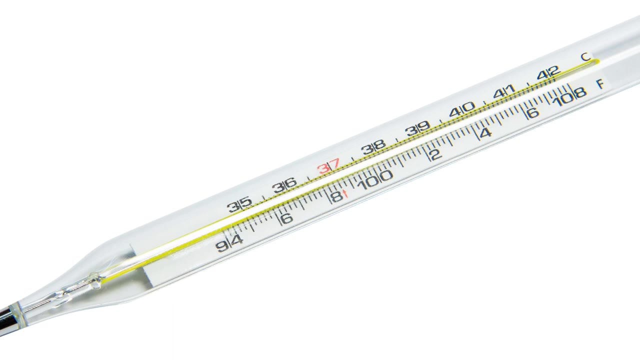 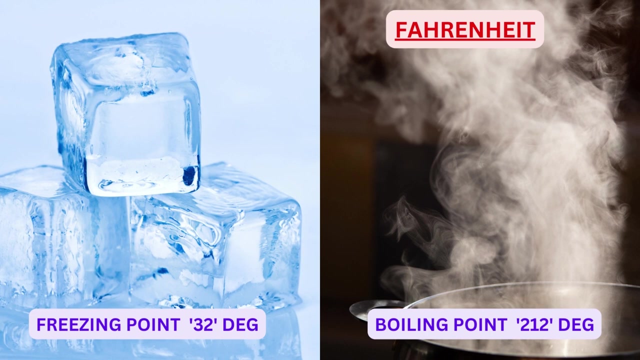 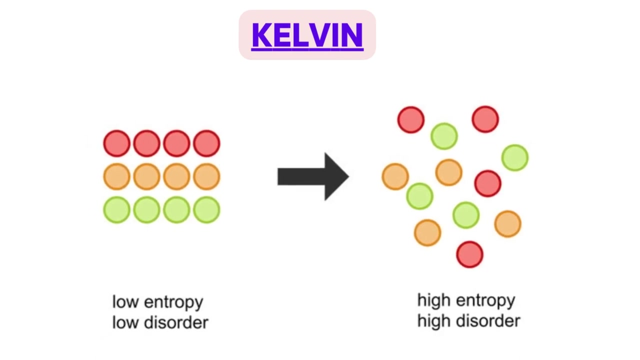 your lifetime, you must have sometime had fever, And fever is measured by mercury thermometer, in Fahrenheit And in Fahrenheit scale. water freezes at 32 degree Fahrenheit and boils at 212 degree Fahrenheit. And what is Kelvin? This scale of temperature measurement has been taken from thermodynamics. 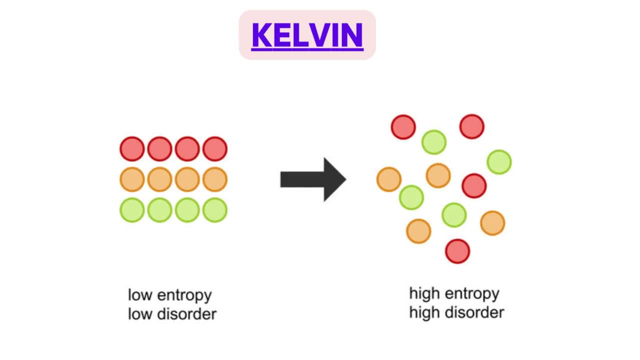 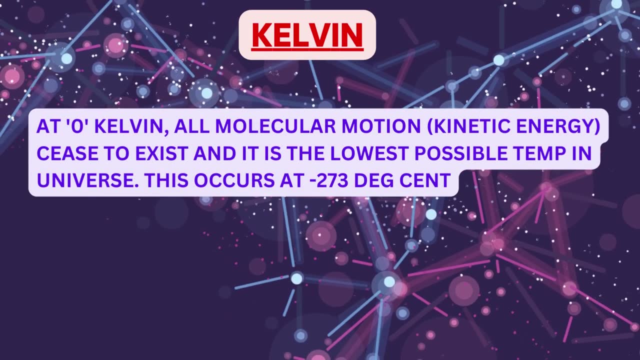 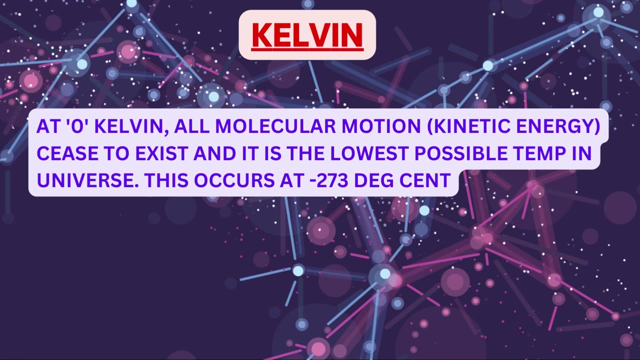 in physics And it is an absolute scale and not relative like degree centigrade and degree Fahrenheit. Since temperature is a measure of average kinetic energy of atoms or molecules, at 0 Kelvin all molecular motion, that is, the kinetic energy, cease to exist And it 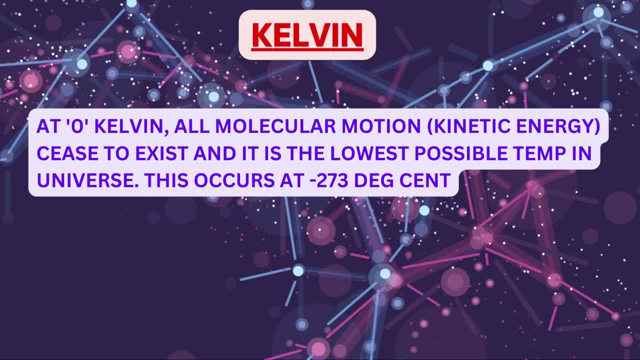 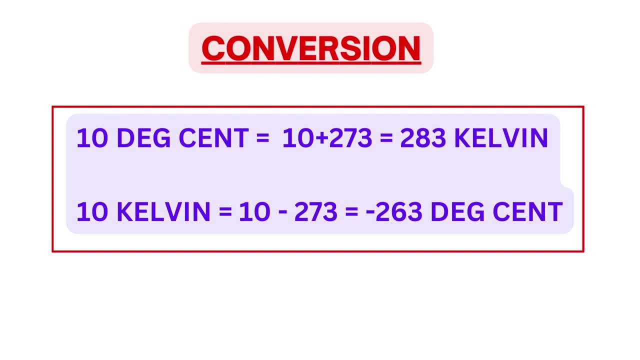 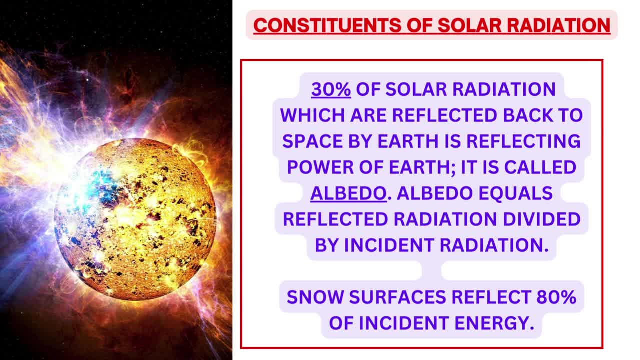 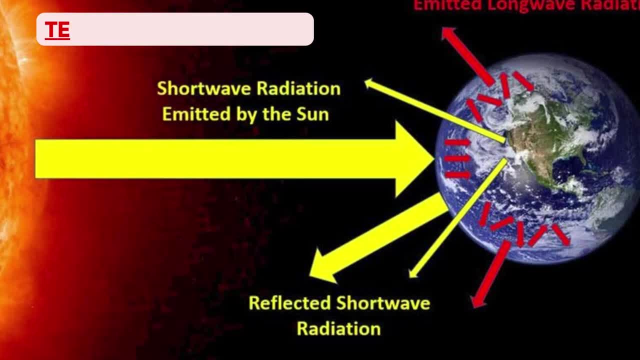 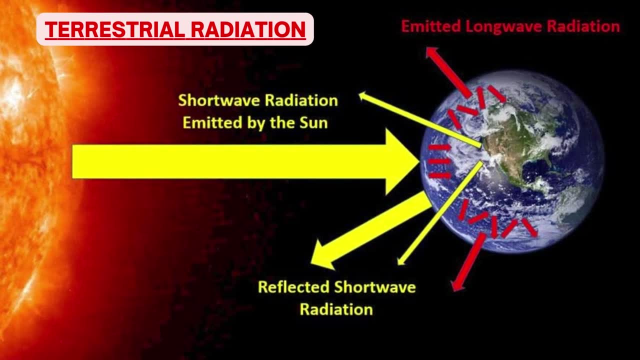 centigrade into Kelvin, just add 273.. For example, if you want to convert degree centigrade divided by incident radiation, Snow surfaces reflect 80% of incident energy- Terrestrial radiation. Once earth gets heated by solar energy or solar insulation. 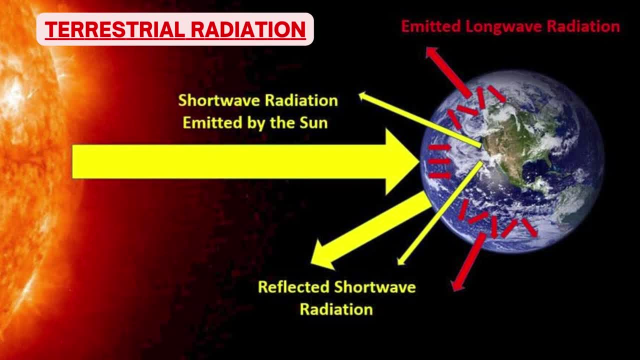 it transmits the heat energy to atmosphere in the form of long wave radiation, and the long wavelength is due to the lesser temperature of the earth surface. Heating of atmosphere from earth's long wave radiation is called terrestrial radiation. What is nocturnal radiation? The cooling of earth surface by long wave radiation. 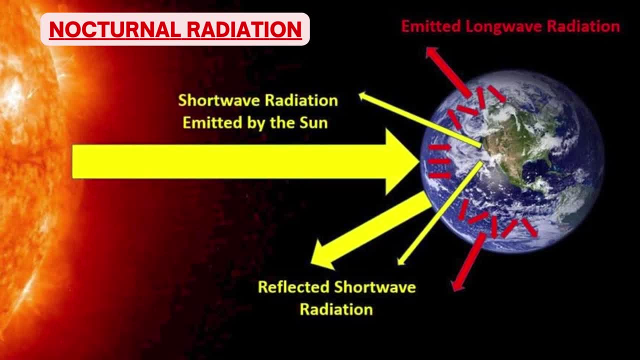 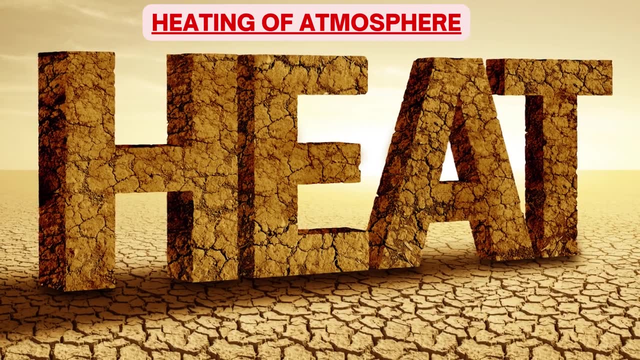 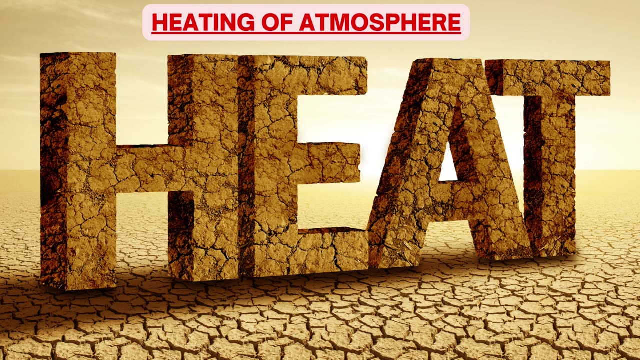 in night is called nocturnal radiation. Heating of atmosphere. It is natural to presume that atmosphere is heated from solar radiation, but that is not true. Atmosphere is transparent to solar radiation and atmosphere gets heated mainly from below, that is, from the atmosphere. Atmosphere gets heated mainly from below. 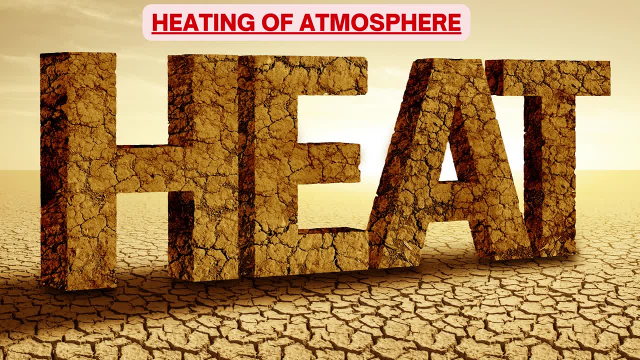 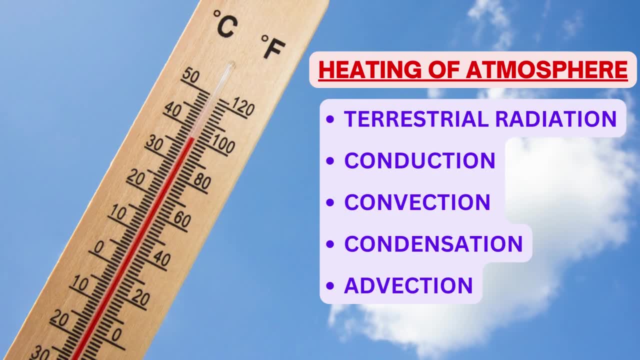 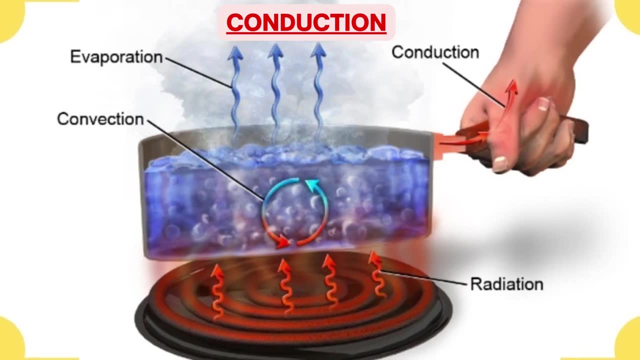 that is, from earth's surface. Atmospheric heating takes place through one of the five ways, which will be described one by one. The first is terrestrial radiation, which we have already discussed. Second is conduction, When you put a utensil on a gas stove to boil. 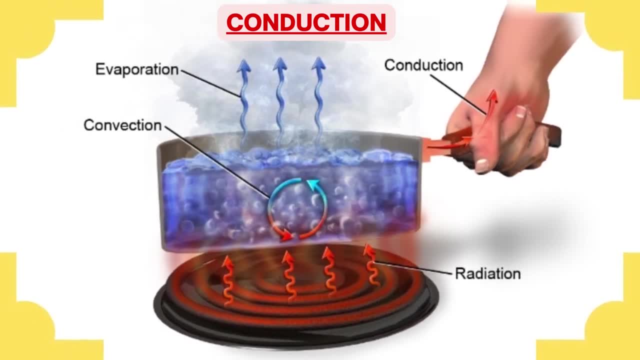 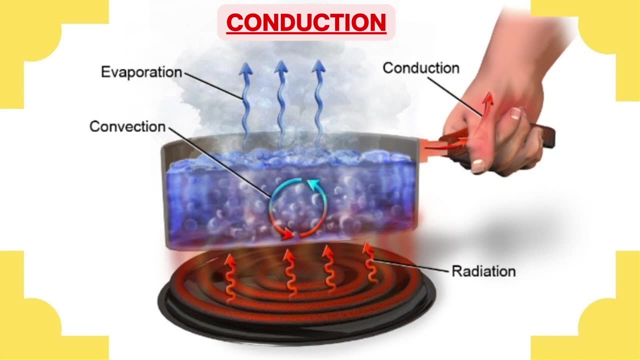 water, the handle of the utensil also gets heated. This is happening since the heat is transferred from one part of the metal to other, through the physical transfer of heat from one atom to another, and so on. This method of heating is called conduction. So when air near the earth, 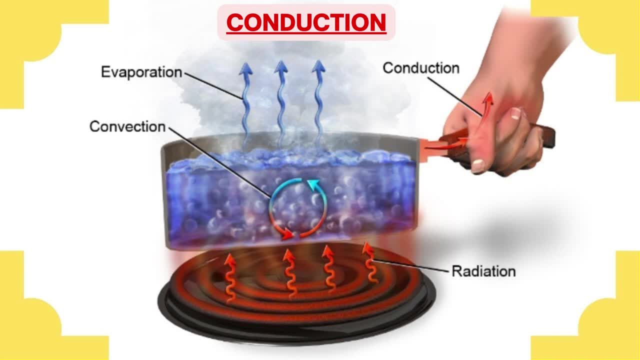 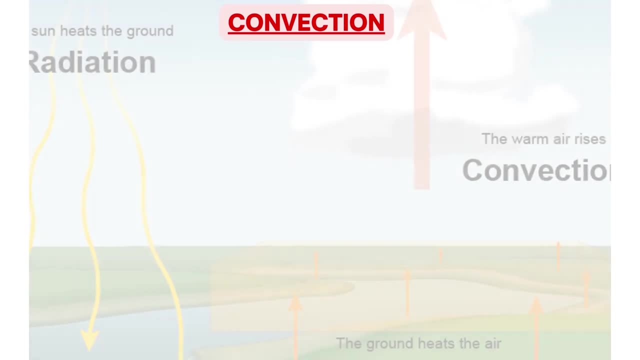 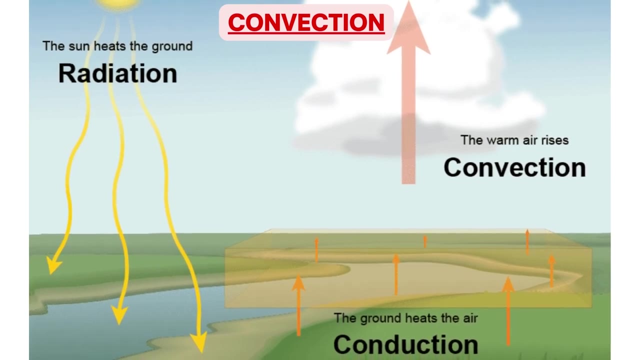 gets heated up. heat is transferred to higher height through conduction, That is, from one molecule to another and to another, and so on. Next is convection. Convection, heating or cooling is when a parcel of material physically moves from one place to another and transfer the heat. 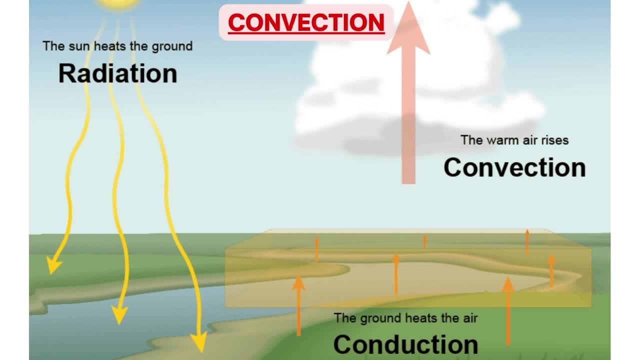 Air near the earth's surface will get heated by conduction, and due to heating, the density will reduce, It will become lighter and therefore it will rise upwards to a higher height in the atmosphere, and then, by doing so, it will transfer the heat to the surrounding. This process is called 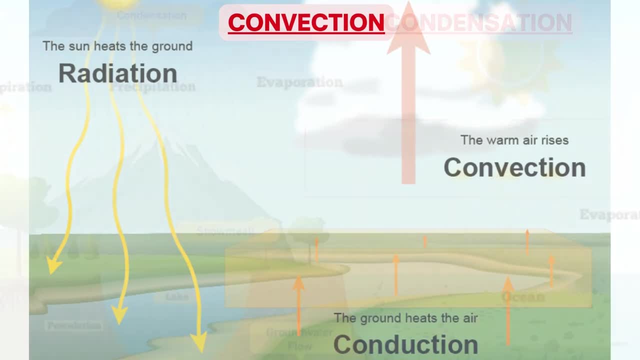 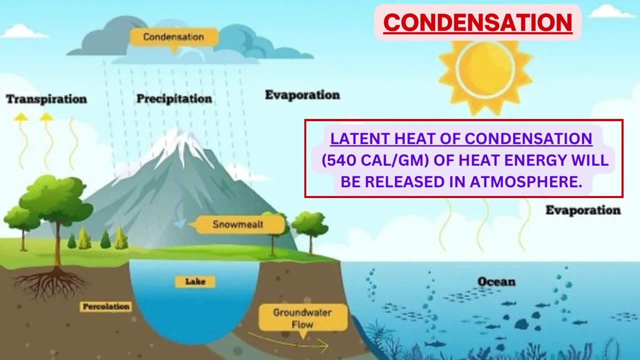 convection Condensation. As the air is lifted, it will be cooled due to the lapse rate of the atmosphere. As the air is lifted, it will be cooled due to the lapse rate of the atmosphere, But when the temperature reduces, the capability of air to hold water vapor will also reduce. 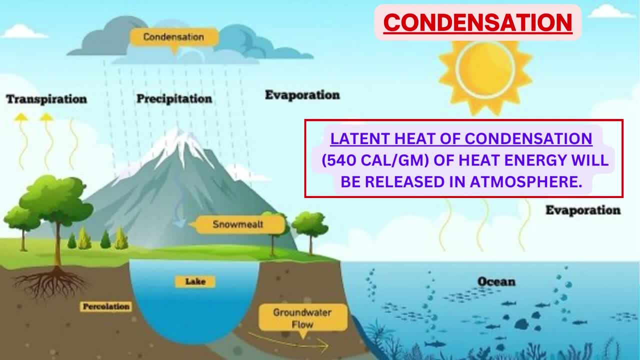 And below a certain temperature, excess water vapor will condense into liquid water. In this process, the latent heat of condensation, and that is 540 calorie per gram of heat energy, will be released into the atmosphere. The last method of heating is advection. 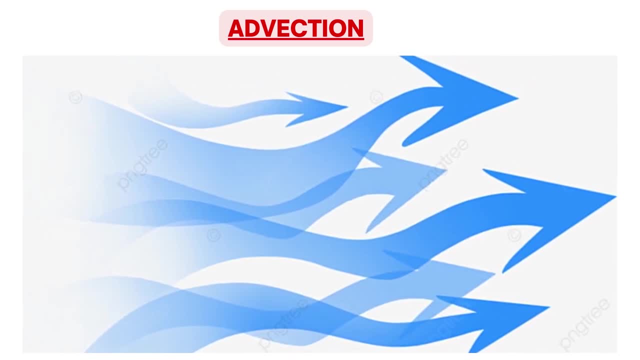 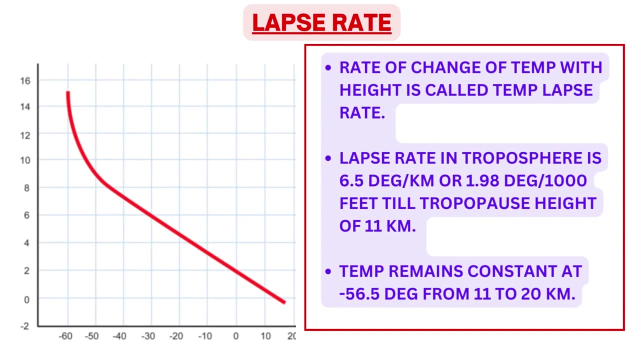 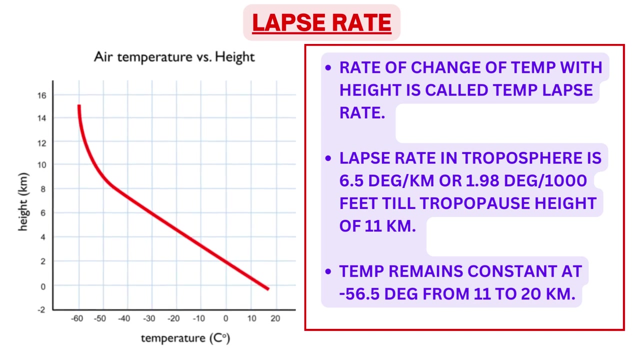 Advection is transfer of heat through horizontal movement of air. Lapse rate: Rate of change of temperature with height is called temperature lapse rate. Lapse rate in troposphere is 6.5 degree per kilometer or 1.98 degree per thousand feet till. 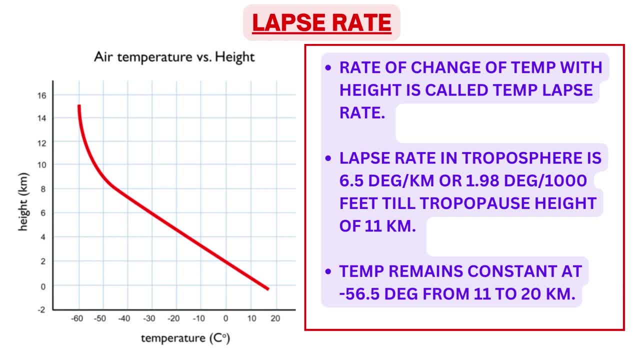 tropopause height of 11 kilometer. Above 11 kilometer, up to 20 kilometer. the temperature remains constant at minus 56.5 degree And you all know that, as per ISA, the mean sea level temperature is considered to be plus 15. 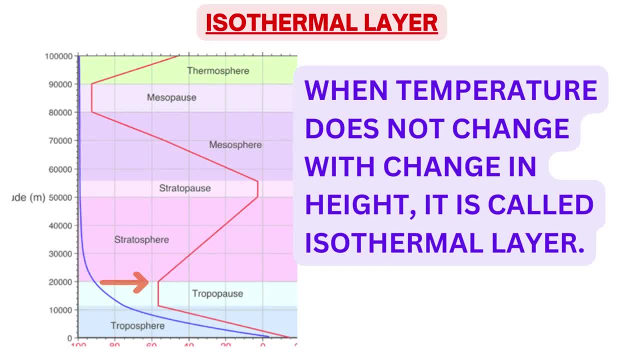 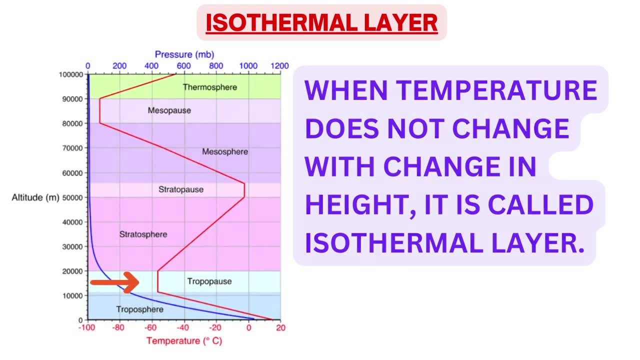 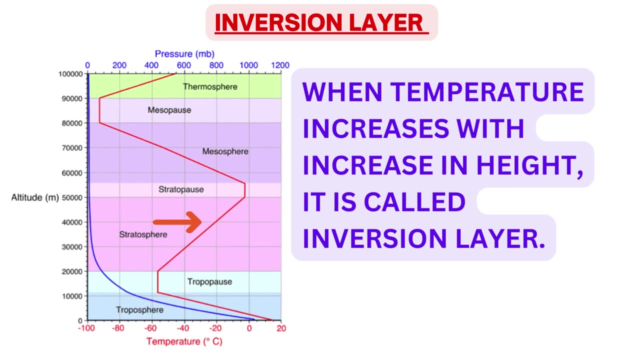 degrees Celsius. Isothermal layer: When temperature does not change with height, it is called isothermal layer. What is inversion layer? When the temperature increase with increase in height, it is called inversion layer. Isothermal and inversion layers are associated with stability. 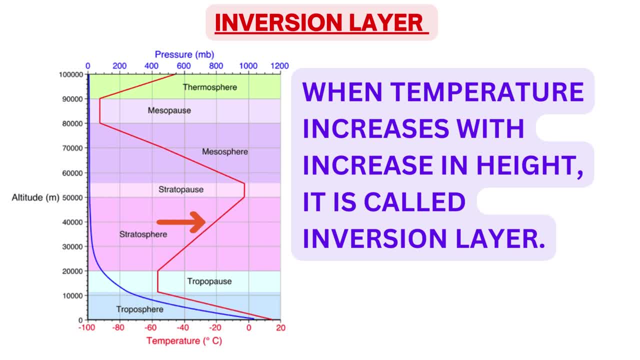 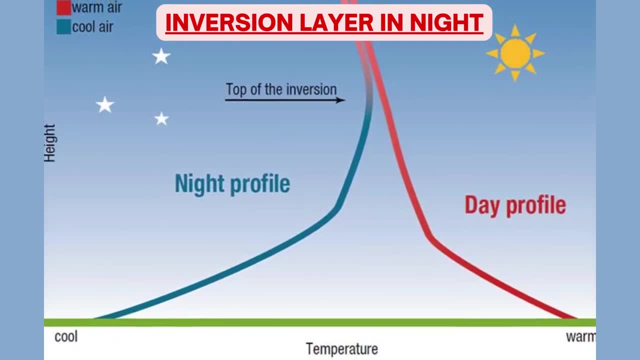 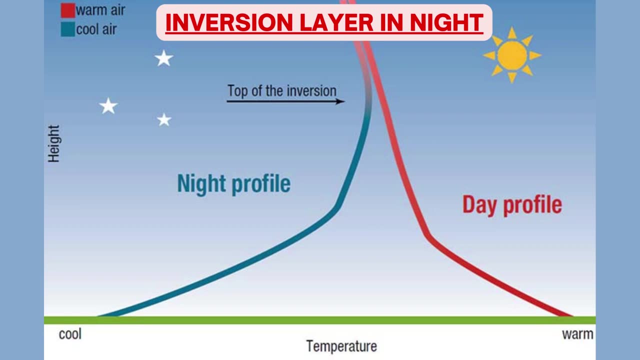 in the atmosphere. This we'll discuss separately in the next video. Inversion layer in night. In night, earth loses its heat energy by radiating heat into the atmosphere. Since there is no solar radiation in the night, earth starts cooling after sunset. 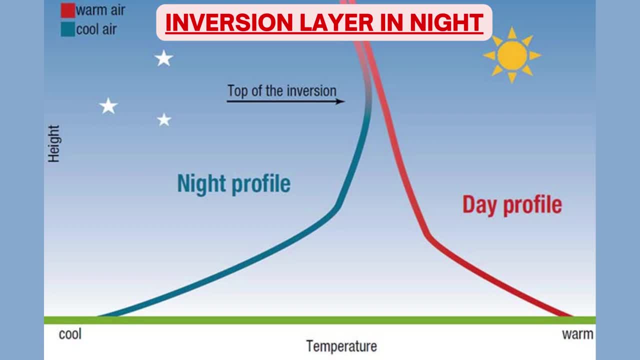 This results in cooler temperature of air which is in contact with the ground below at night. Generally, the height of this layer is 1 kilometer above the ground, Whereas the temperature of air above 1 km is still warm in night. So this results in the presence of inversion layer near the ground at night, wherein the air at a lower height is cooler as compared to air at a higher height. 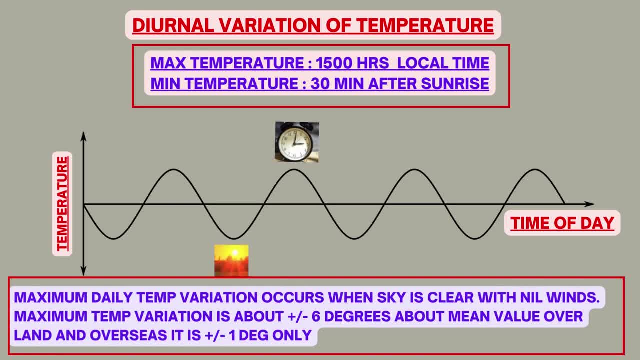 Durable variation of temperature. Daily change recorded at a given place between maximum and minimum temperature over 24 hour cycle is called diurnal variation of temperature. Maximum local temperature is recorded at 1500 hours in the afternoon and minimum temperature is recorded half an hour after sunrise. 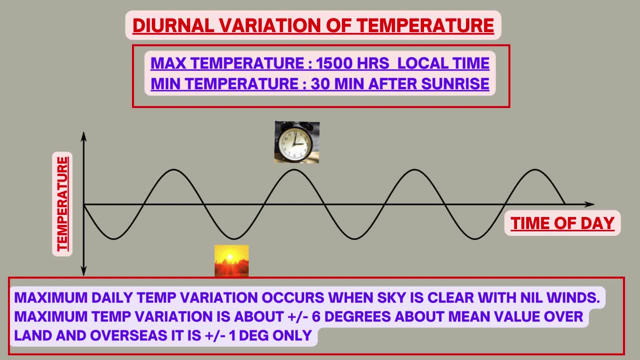 Maximum daily temperature variation occurs when sky is clear, with nil winds or light winds, And maximum temperature variation is about plus minus 6 degree about the mean value. over the land and overseas, the diurnal variation of temperature is hardly plus minus 1 degree about the mean value. 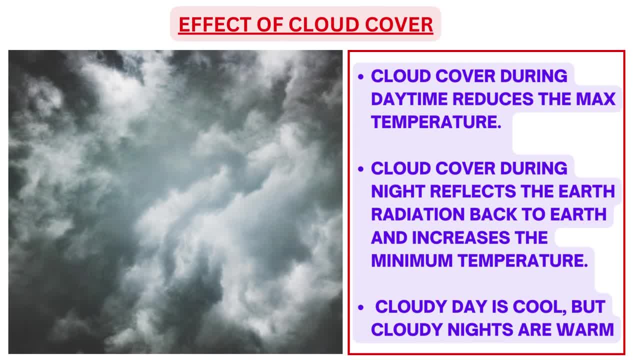 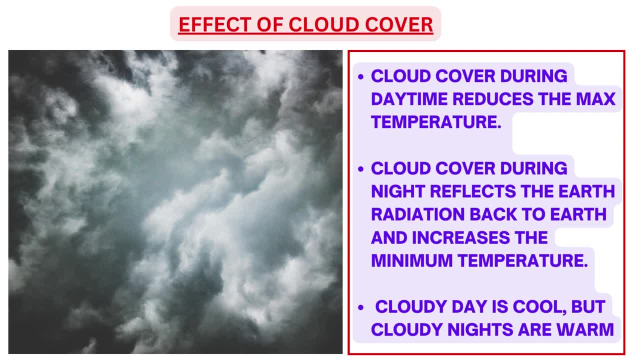 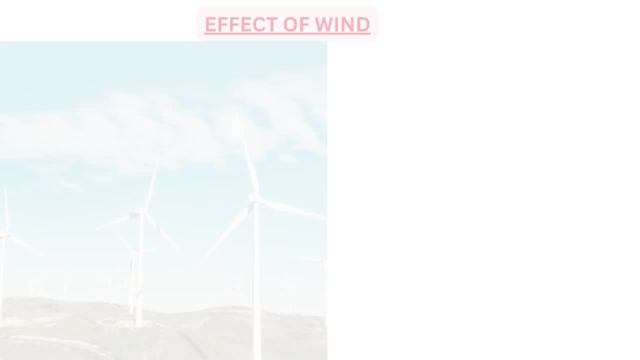 Cloud cover. Cloud cover during day time reduces the maximum temperature. The cloud cover during night reflects the earth radiation back to earth and increases the minimum temperature. So the cloudy day is cool, But the cloudy nights are warm. Effect of wind: By day the wind will cause the maximum temperature to reduce. 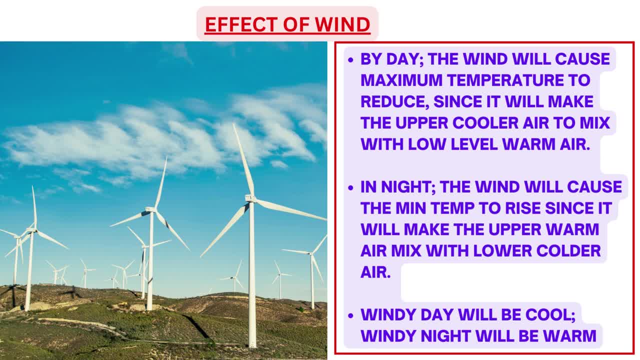 Since it will make the upper cooler air mix with the low level warm air. In the night, the wind will cause the minimum temperature to rise, Since it will make the upper warm air mix with the lower, colder air. So, to summarize, the windy day will be cool and windy night will be warmer. 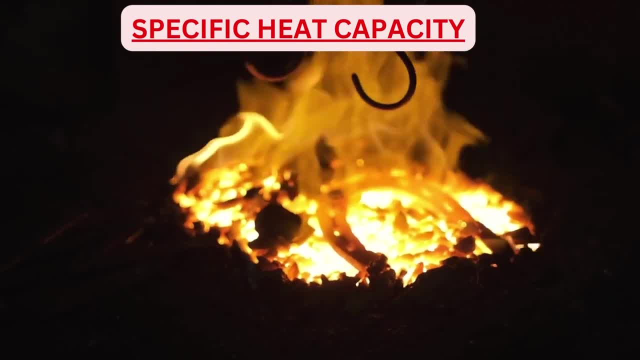 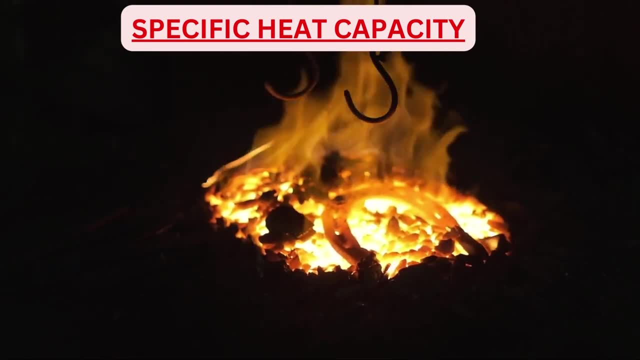 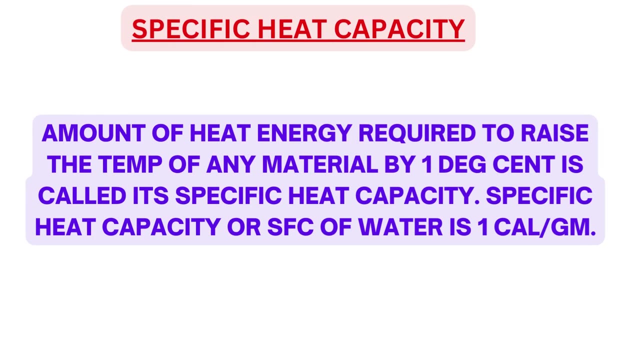 Specific heat capacity. To heat up any material or, to be precise, to raise the temperature of any material, we need to supply heat energy to it. The amount of heat energy required to raise the temperature of any material by 1 degree centigrade is called its specific heat capacity. 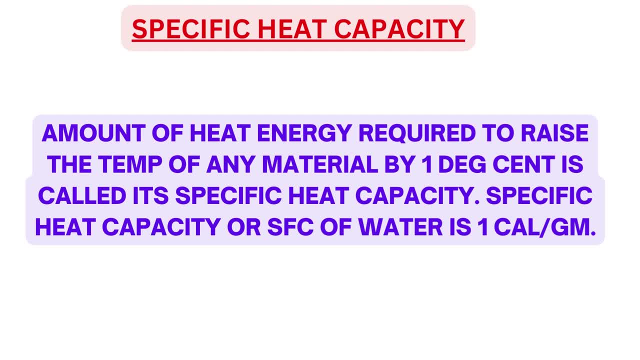 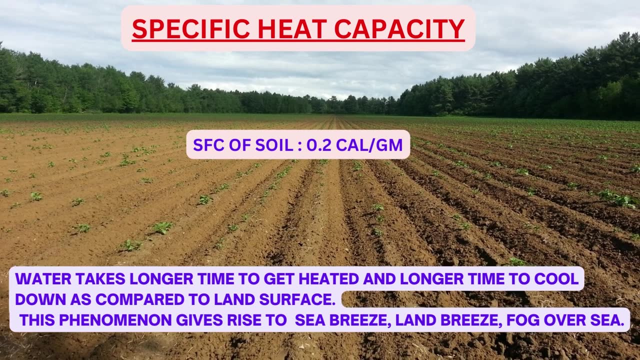 Specific heat capacity, or SFC, of water is 1 calorie per gram. It means 1 calorie energy is required To raise the temperature of 1 gram of water by 1 degree centigrade. Specific heat capacity of soil on earth is decimal 2 calorie per gram. 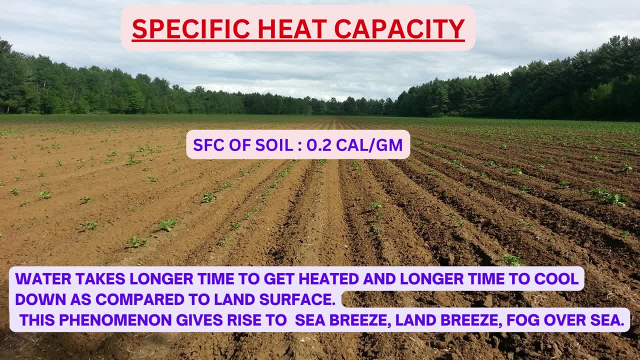 That means it will require 5 times more energy to raise the temperature of water by 1 degree as compared to soil on earth. To summarize, the water takes longer time to get heated and longer time to cool down. as compared to land surface, This phenomena gives rise. 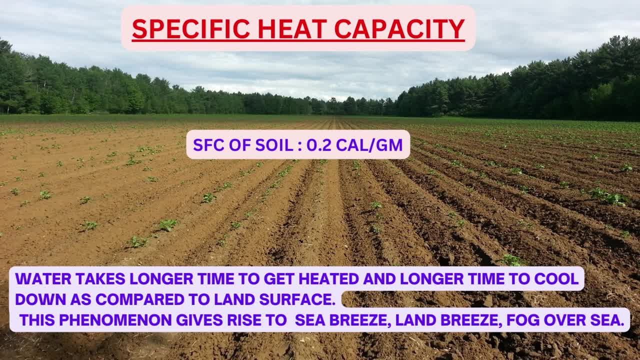 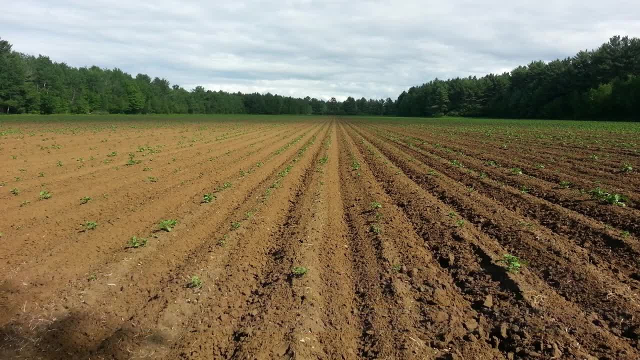 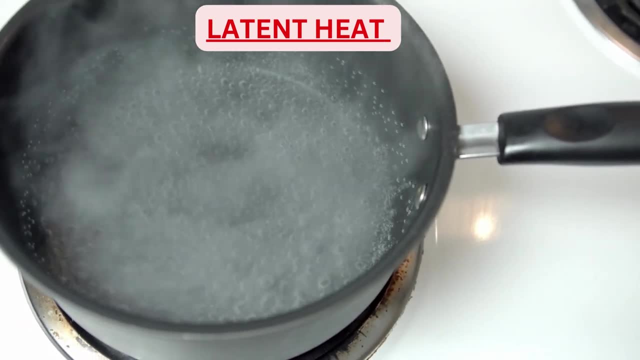 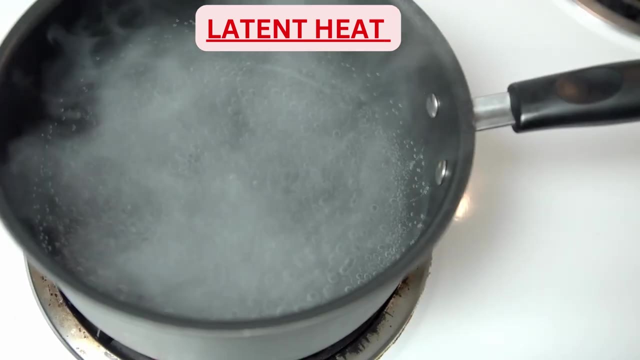 To many situations like sea breeze, land breeze, fog over sea, etc. Latent heat. Latent means hidden And latent heat means hidden heat. Let us understand this with an example. When we boil water, it gets heated up and at 100 degree centigrade it starts boiling. 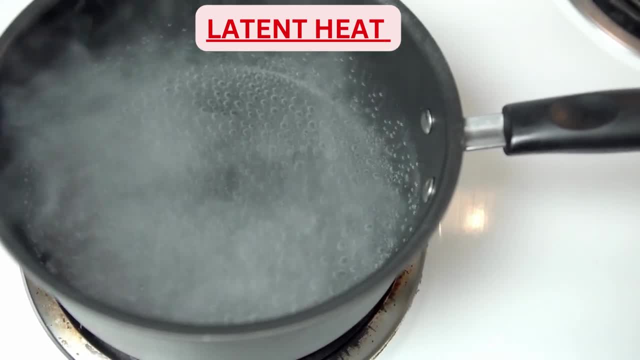 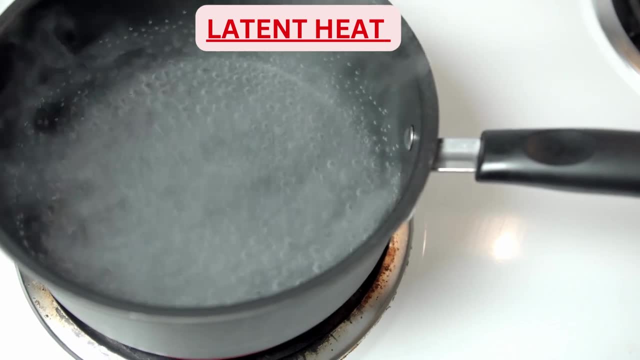 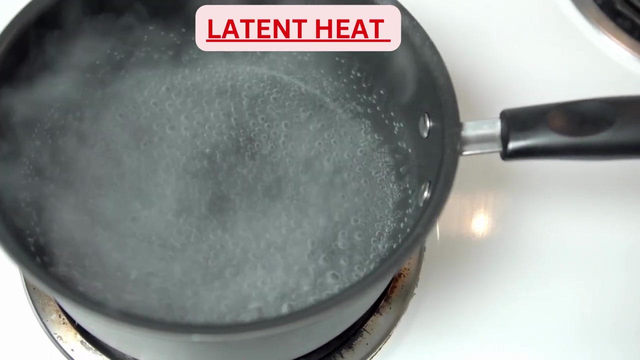 At boiling point. if we put a thermometer in the utensil, We will observe that the temperature Of boiling water will remain 100 degree, no matter how long you boil it. So where is the heat energy of the gas stove going? Well, at boiling point, liquid water is converting into the gaseous water vapor. 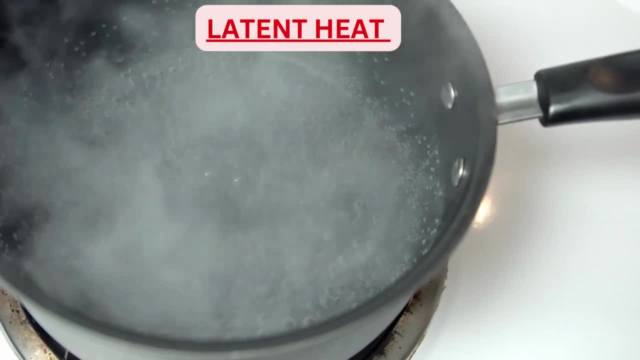 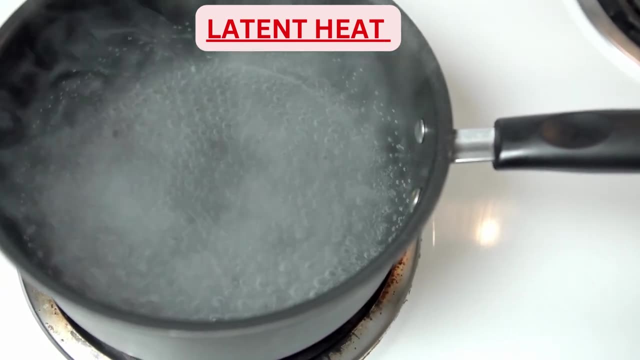 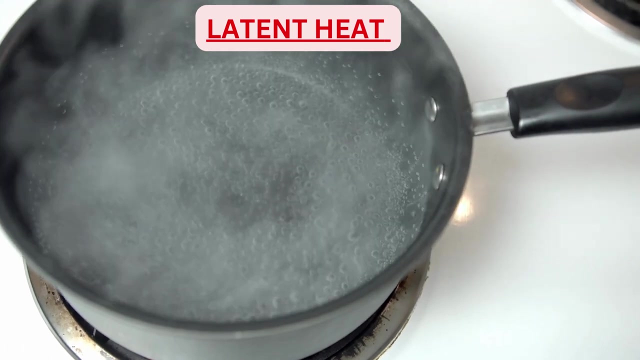 Conversion of liquid water to water vapor requires heat energy. So liquid water is converting to water vapor with no change in temperature, but consuming some amount of heat energy. This is what is called latent heat or hidden heat. The latent heat of vaporization of water is 540 calorie per gram. 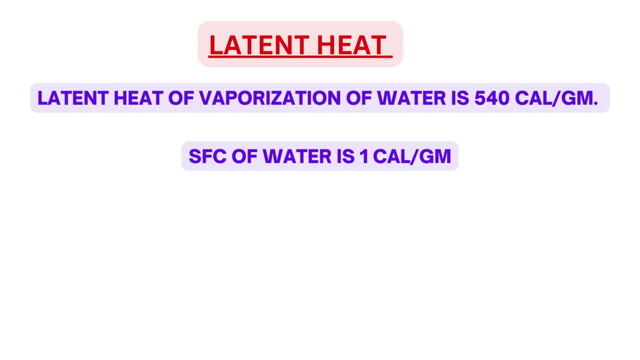 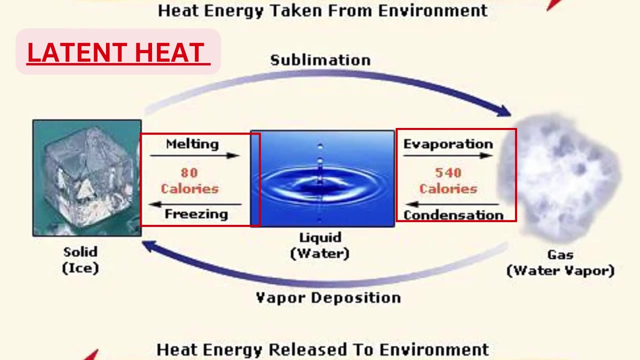 That means it will require 540 more times of heat energy to vaporize 1 gram of water, as compared to changing the temperature by 1 degree centigrade of 1 gram of water, which is a huge difference. So you see, when water vapor condenses back to liquid water, it will release the same amount of heat energy back into the atmosphere. 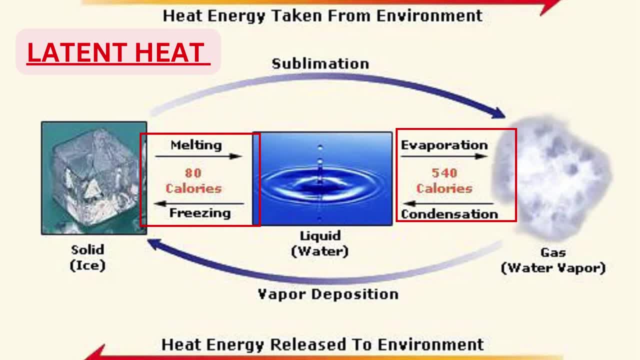 Atmosphere. Atmosphere also gets heated up through release of this latent heat whenever the condensation of water vapor takes place into the liquid water. The latent heat required to melt solid water, that is, ice, into liquid water at 0 degree centigrade is 80 calorie per gram. 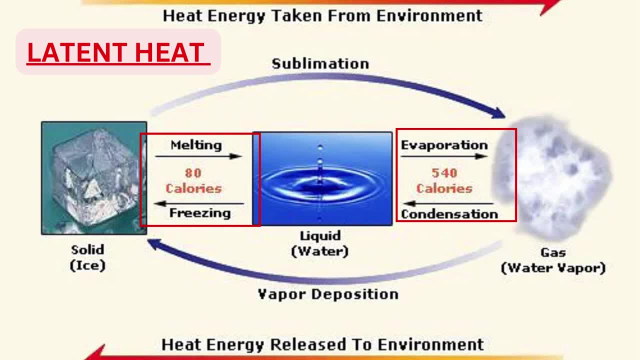 And when the liquid water gets converted to ice- and that is what happens in your refrigerator- it will release 80 calorie of heat per gram of water. And this Released heat is released into the atmosphere through the backside of your fridge, and that is why the backside of the fridges which is kept in our home feels quite warm and hot. 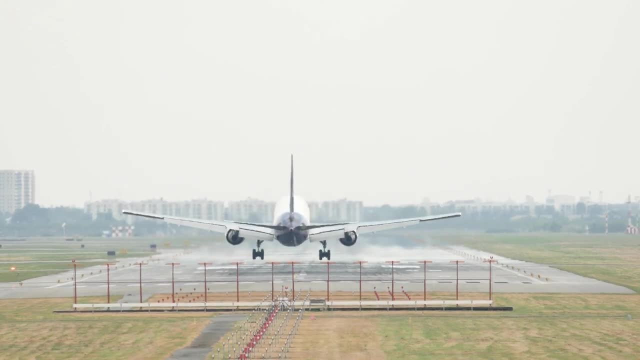 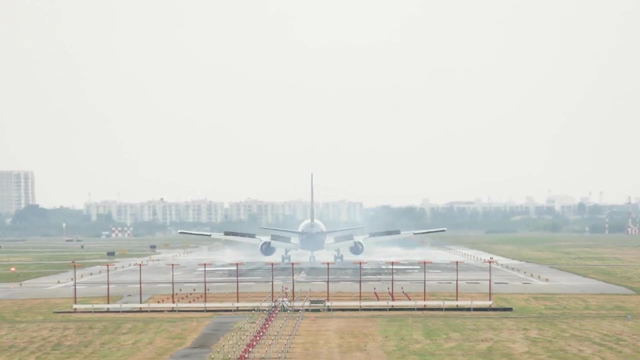 So hope this video has helped you in understanding the subject temperature in the meteorology. With this we have arrived at our destination. hope to see you on board again for the next flight. like, share, subscribe and comment if you wish. happy landings. Thanks for watching.